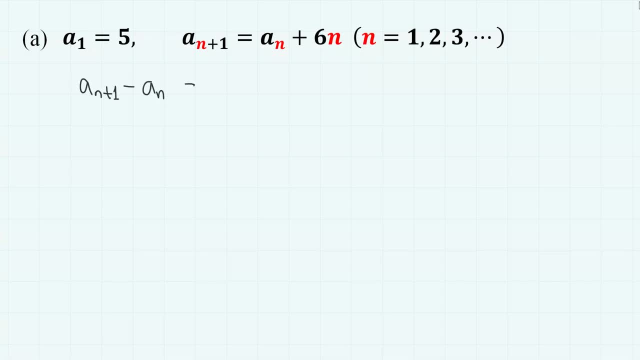 the difference an plus 1, minus an is given as 6.. Now let us substitute n equals 1,, 2,, 3, and so on all the way up to n minus 1, to see what happens. When n equals 1, we have a2 minus a1 equals 6 times 1.. And when n equals 2, we have 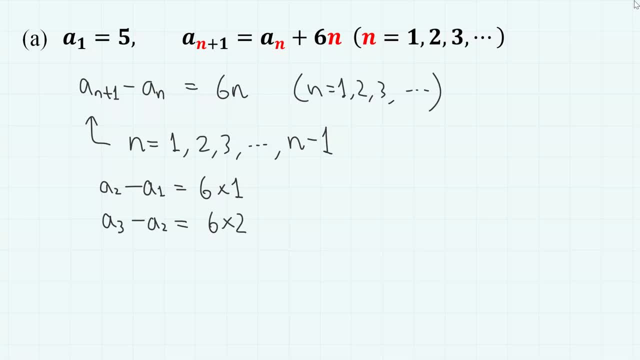 a3 minus a2 equals 6 times 2.. And when n equals 3, we have a4 minus a3 equals 6 times 3, and so on. And finally, when n equals 3, we have a3 minus a1 equals 6 times 3.. And so on. 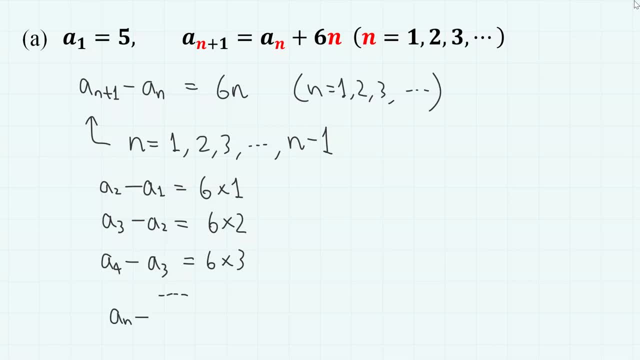 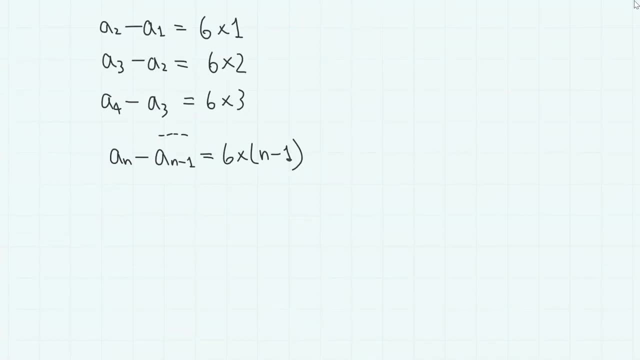 for n equals n minus 1, we have a n minus a. n minus 1 equals 6 times n minus 1.. Now notice that if we add them up, we have a 2 cancelled out and a 3 cancelled out. 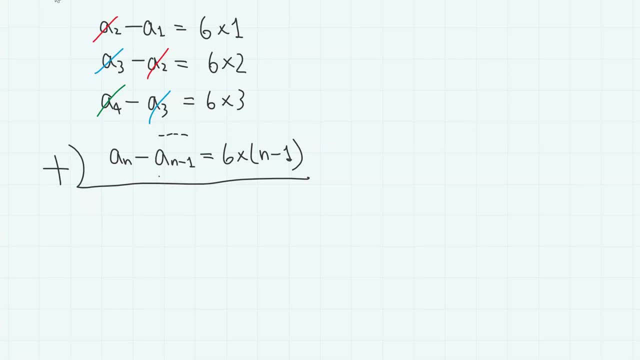 and a 4 cancelled out, and so on, And for the last part we have a n minus 1 cancelled out. So on the left-hand side we are left with a n minus a 1, and on the right-hand side, 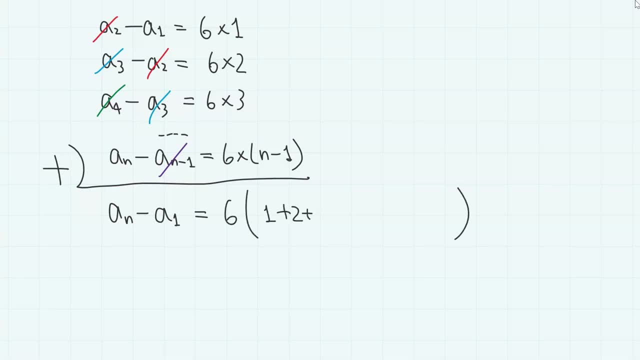 we have 6 times 1 plus 2 plus 3 plus, so on till plus n minus 1.. Here it is given that a 1 equals 5, and using the formula for the sum of natural numbers, we have a n equals 5 plus 6 times n. 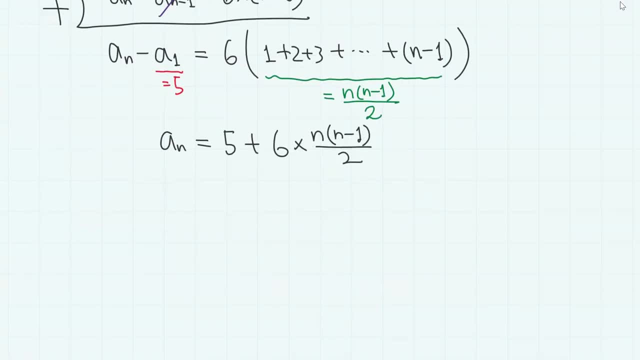 n minus 1 over 2, which is 5 plus 3 n squared minus n. So we have a n equals n minus 1.. 3 n squared minus 3 n plus 5.. And this is the answer For the second problem. we do the same, But first let us simplify the expression for the. 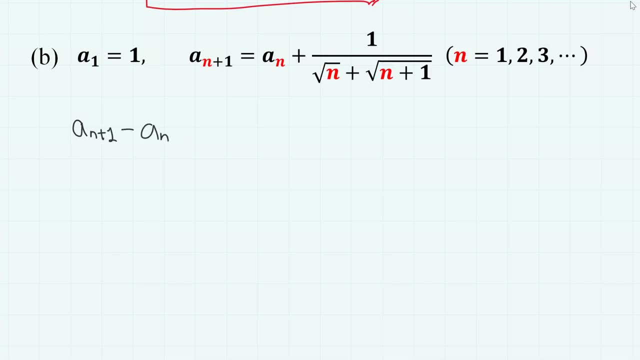 difference a n plus 1 minus a n a little bit, which is 1 over square root of n plus square root of n plus 1.. We rationalize the denominator by multiplying square root of n plus 1 minus square root of n. 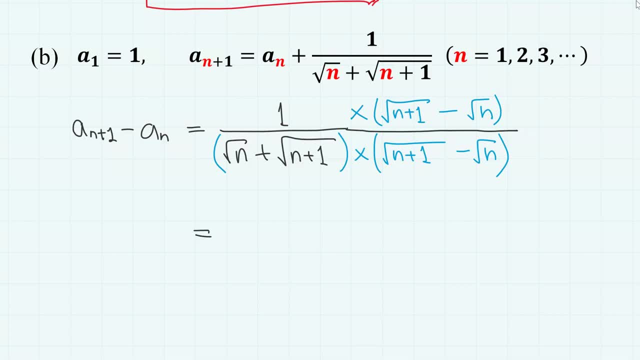 Then, on the numerator, we have square root of n plus 1 minus square root of n, And on the denominator, we simply have n plus 1 minus n. So we simply have square root of n plus 1 minus square root of n. So we have this. And substituting n with 1 to 3. dot, dot, dot. 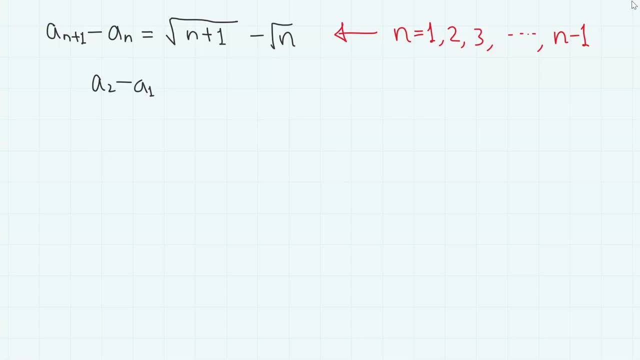 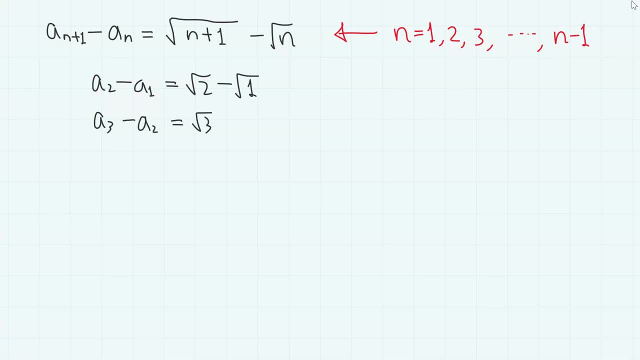 denominator. we have a 2 minus a 1 equals square root of n plus square root of n, And on the 3 minus a 2 equals square root of 3 minus square root of 2, for n equals 2, and we have this and so 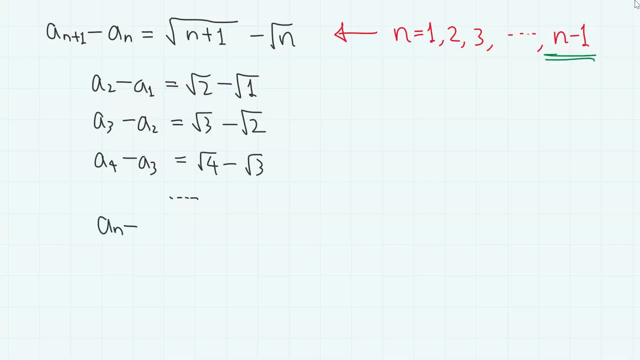 on. and for the last one, we have a n minus a n minus 1 equals square root of n minus square root of n minus 1.. if we add them up on the left hand side: a 2 cancel out. a 3 cancel out. a 4 cancel out. 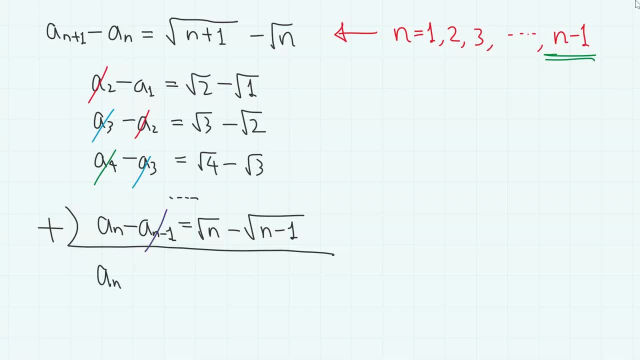 and a n minus 1- cancel out. so we have a n minus a 1 and on the right hand side, square root of 2- cancel out, square root of 3- cancel out, square root of 4- cancel out. and square root of n minus 1- cancel out. so we have square root of n minus square root of 1 and it is given that a 1 equals. 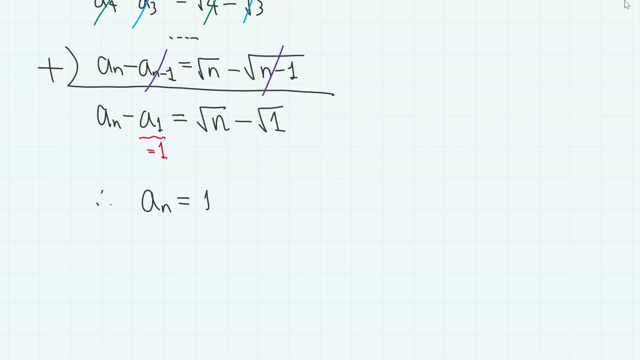 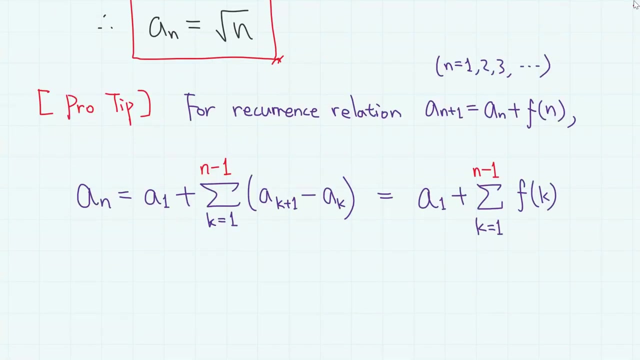 1, so we have a n equals 1 plus square root of n, minus square root of 1, so we have a n equals square root of n. And this is the answer for the second problem. In general for recurrence relations, given as a n plus 1 equals a n plus f n, we can find the general. 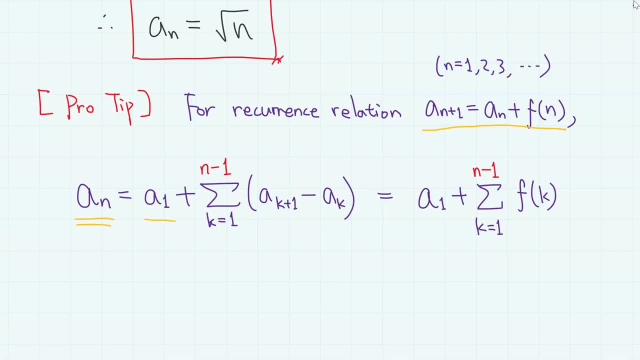 expression for the nth term by a 1, the first term plus we add up the difference between adjacent terms: a k plus 1 minus a k. from k equals 1 to n minus 1.. Remember that this part must be n minus.